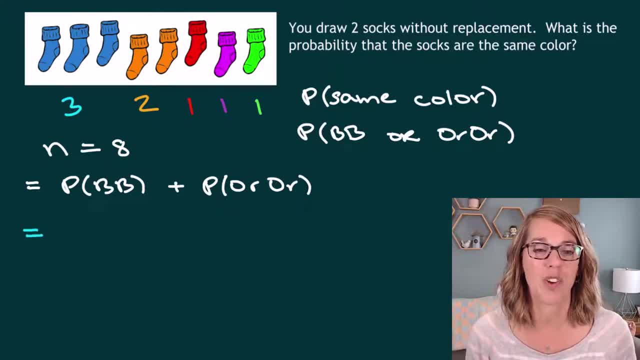 case. first, I want the probability of drawing that first blue sock. I go back up and I look at my socks. There are three different blue socks that I have to choose from. So that gives me three favorable outcomes out of the total Eight. But I'm going to take one of those blue socks, I'm going to draw it out and put it aside. 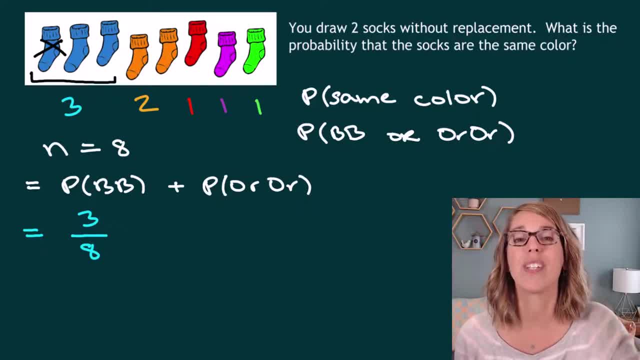 Now I'm looking for the probability of blue and a blue. So now I'm going to go back in and I'm drawing for that second blue sock. Well, there are two blue socks remaining, So that's going to be times two. And there are. I've got one less sock, right, So I've got one, two, three, four, five. 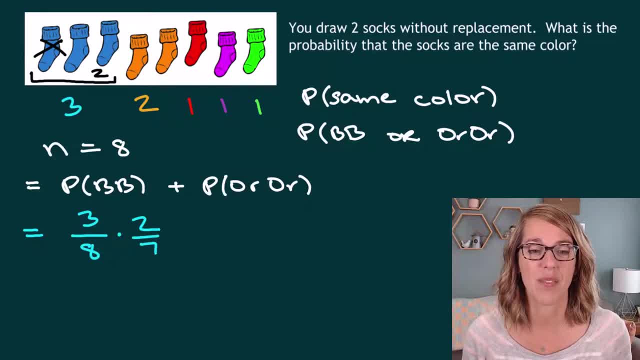 six, seven socks remaining, So seven goes in my denominator. Now I'm going to go back to the drawing board or back to the full drawer of socks and grab orange socks. So as I'm trying to grab orange socks, there are two orange socks to choose. 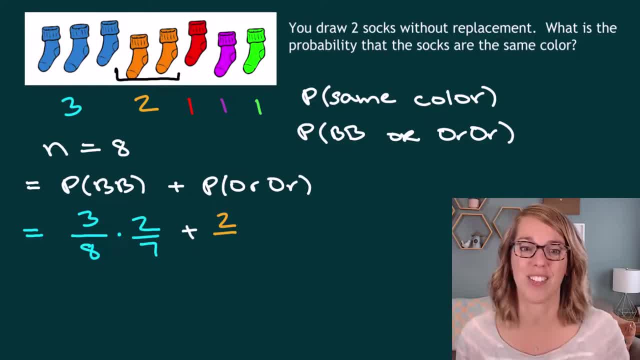 from to start. So there are two, and all eight socks are back in the drawer. We're starting this new case fresh, So that would be orange, and so I'm going to multiply in orange. but I've drawn that first orange sock So that one's gone, which leaves me with a single orange sock out of the 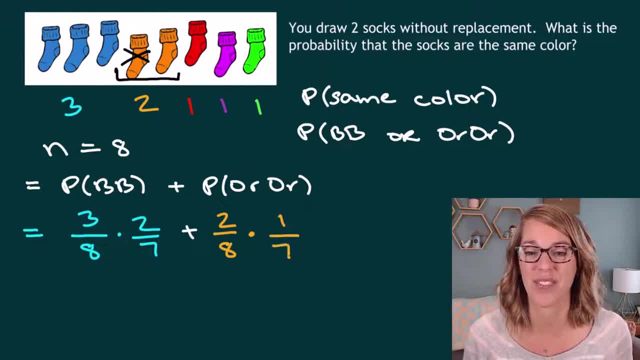 seven that remains, So I've got one out of seven. Now I can do a little bit of math and clean this up. Cancel the twos and I get a four here. Cancel some twos and I get a four here. So I end up with: 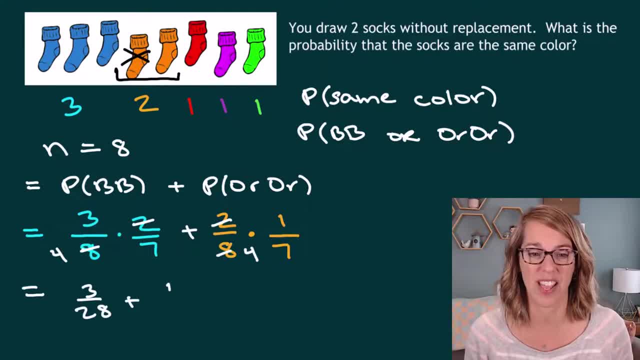 three twenty-eighths plus one twenty-eighth, one twenty-eighth, And that is equal to four twenty-eighths. I can cancel a four out of both the numerator and the denominator and I end up with one seventh expressed as a fraction. 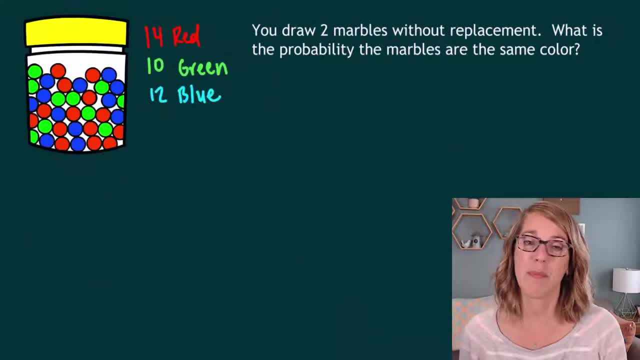 Let's do the marble example next. In my marble example I'm going to be doing the same thing, drawing two without replacement. So one marble gets set aside. I go back and draw the second marble and I'm trying to get a matching. 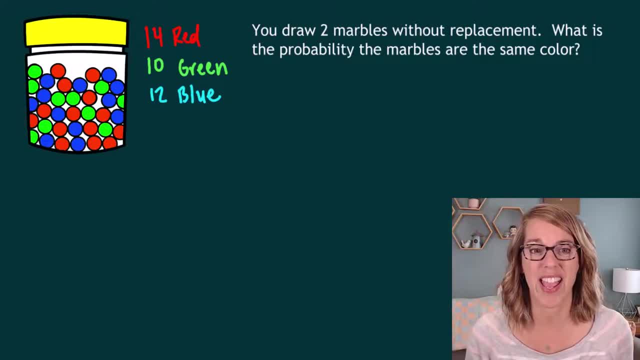 pair. So I've got fourteen red, ten green and twelve blue. How many do I have altogether? So this is thirty-six marbles altogether. We're going to call that n. So this is the probability, again of the same color. 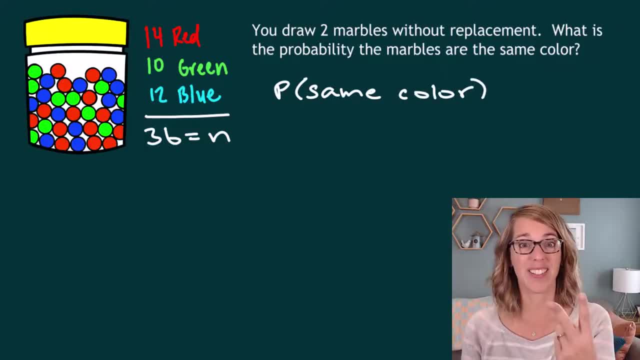 But now I can use two reds together, I can get two greens together, or I can get two blues together. So this would be the probability of red, red, or which we know. we can add the probability of green, green, or so again, we're going to add the probability of blue, blue. 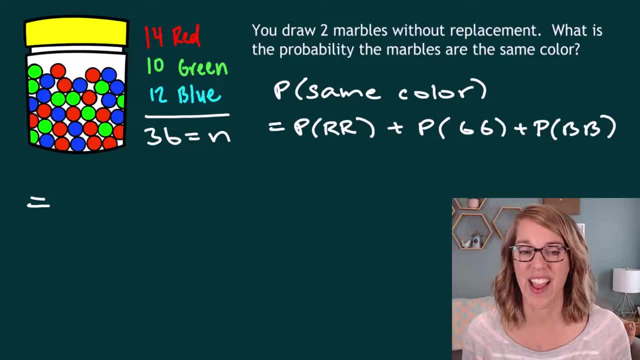 Let's start off with the two reds. I'm going to put this together as a fraction favorable. out of total are 14 red marbles in that jar, So there are 14 ways that I could choose a red marble, So 14 out. 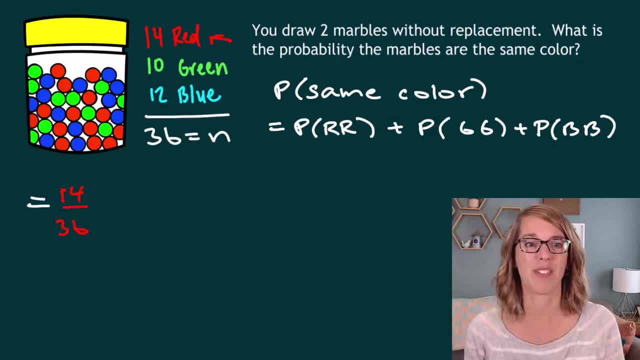 of the 36 total. But this is without replacement, So I'm going to cross off one of those red marbles. It has gotten set aside, So I want red and red, So I'm going to multiply those together. There are now 13 left in this jar, 13 red marbles, Total marbles, because I took that one out. 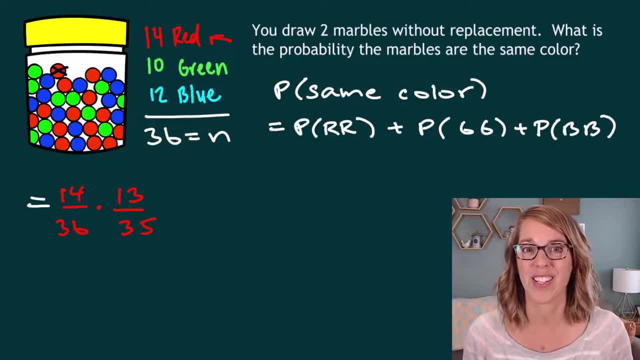 there are 35. So that's our first case- red and red- Or next we're going to do green and green. I want to go back to the full jar, So I've got all 36 in there and I want to start by drawing. 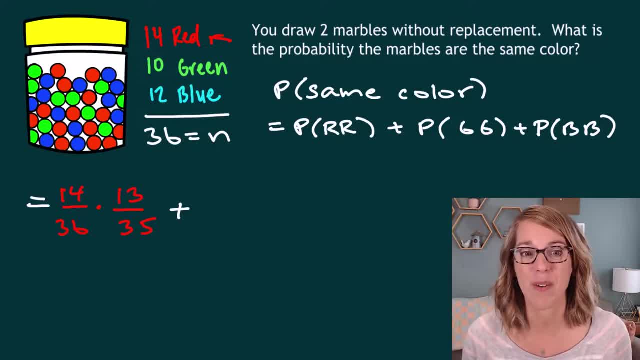 a green marble. Well, there are 10 green marbles to choose from, So there's 10 out of the 36 marbles total. But again, this is without replacement, So I'm taking one of those and setting it aside. 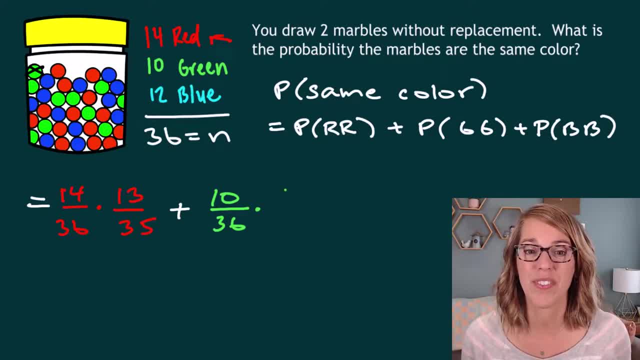 So when I go back to draw that second green marble, there are nine left out of the 35.. Okay, last but not least, we've got those two blue marbles. I again want to go back to a full jar. Now let's go ahead, and 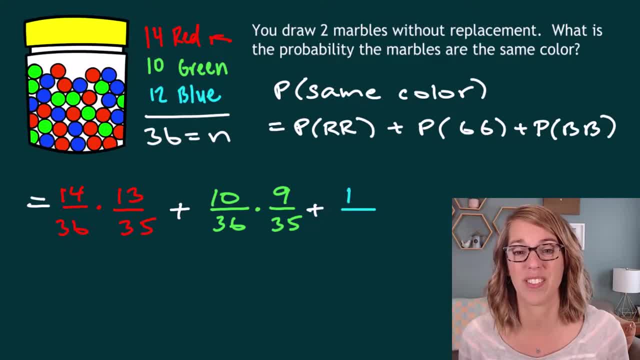 draw some blue. There are 12 blue marbles to start with, So I can draw any one of the 12 to start and all 36 are in the jar. So any 12 out of the 36 times, but I've drawn one out.